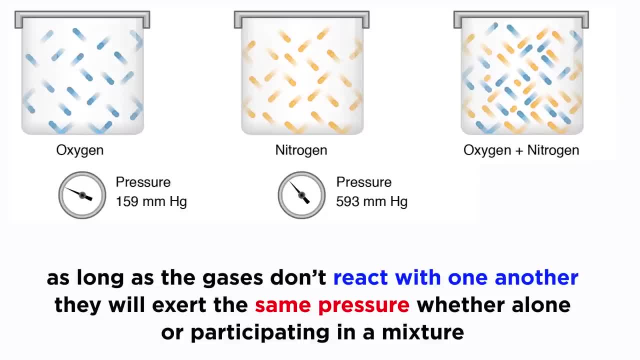 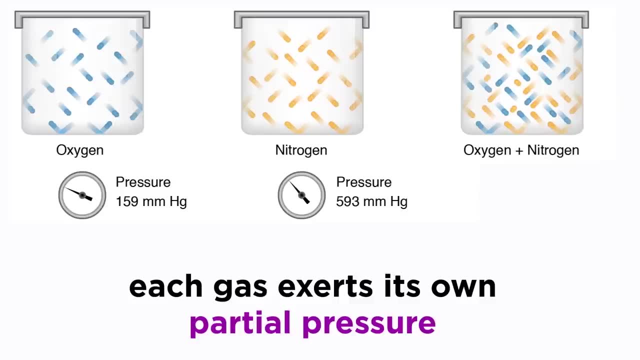 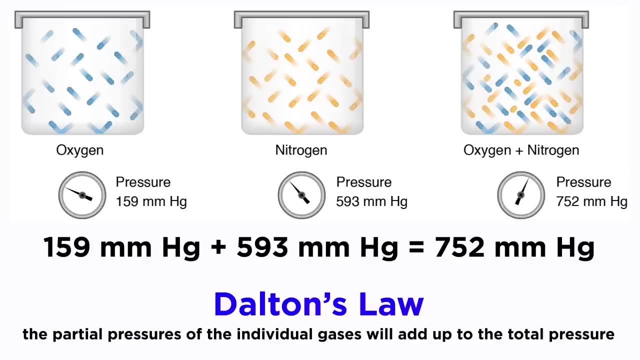 When a mixture of gases is specific to the amount of that particular gas that is present and we will call the pressure of that particular gas its partial pressure. In order to find the total pressure of the vessel, we will simply add up the partial pressures. 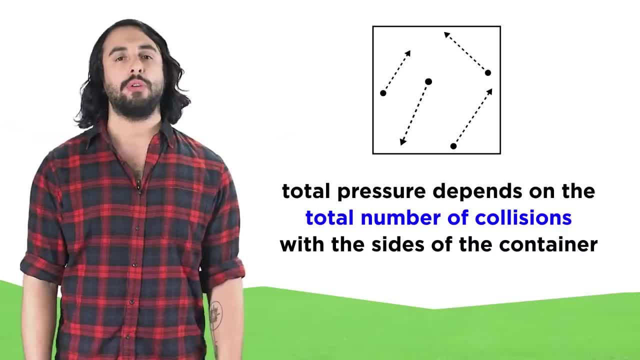 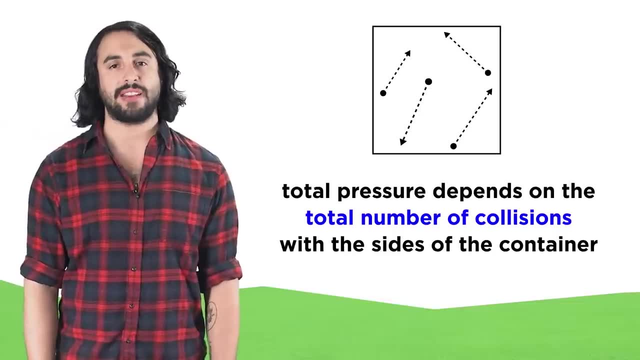 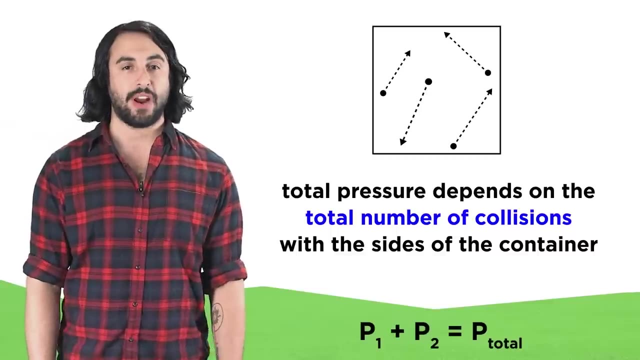 This is stated in Dalton's Law. When you think about it, it makes perfect sense, since pressure is just the force exerted as particles strike. Particles strike the sides of the container. So the pressure from all the particles of one gas plus the pressure from all the particles 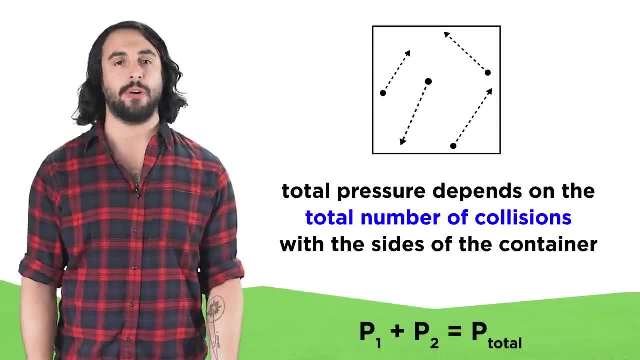 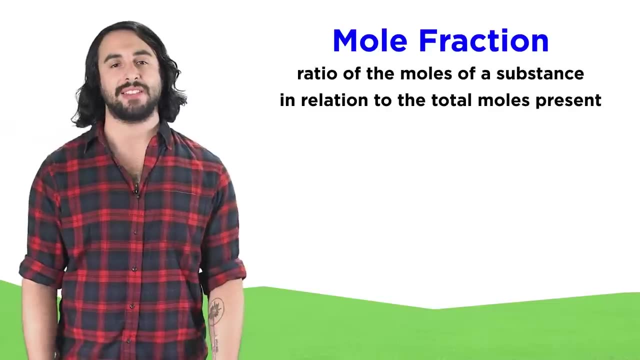 of another gas should add up to be the total pressure for all the particles. assuming we are treating these as ideal gases where their identities are irrelevant, We can also make statements about the partial pressure of each individual gas as they relate to something called the muon. 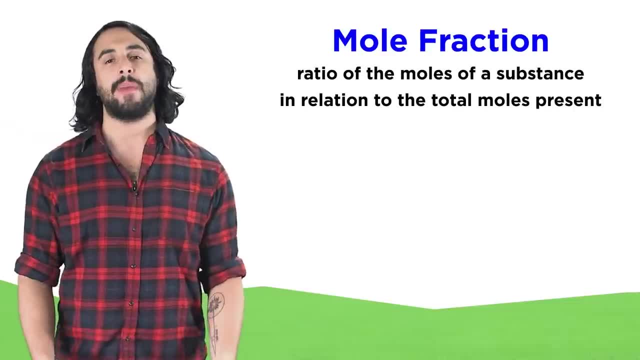 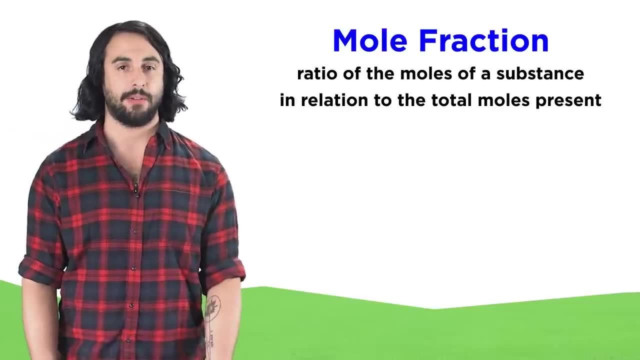 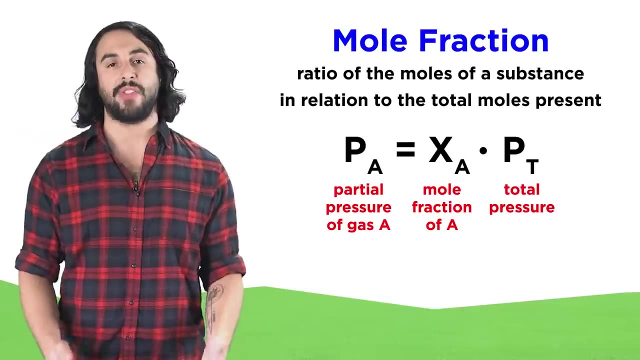 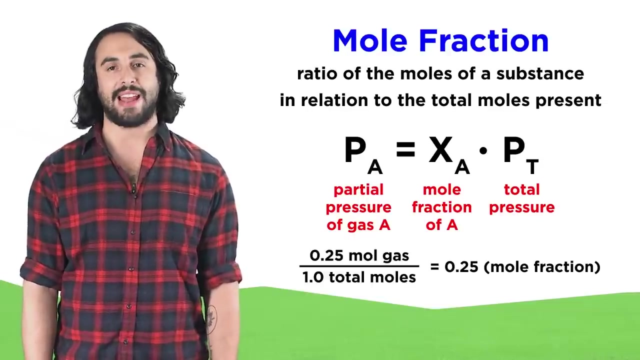 The muon is the number of moles of a substance compared to the total moles of matter present, and the partial pressure of a gas within a mixture will be equal to the mole fraction of that gas times the total pressure. So if there were 0.25 moles of a particular gas out of 1 mole of total gas particles, 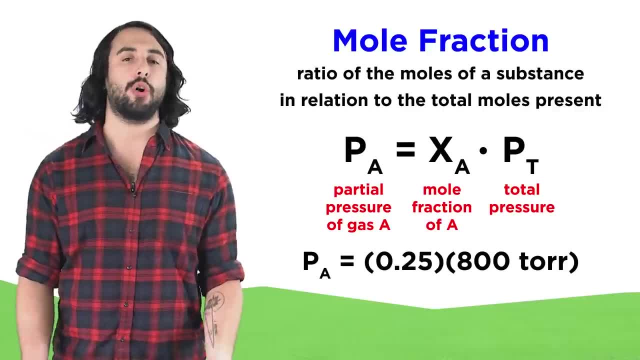 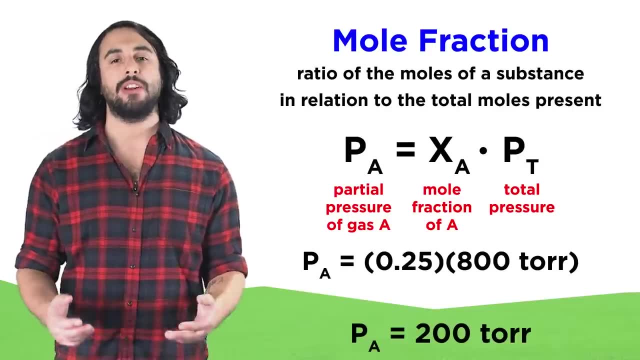 that would mean 0.25 moles of a particular gas out of 1 mole of total gas particles- fraction of 0.25, and if the total pressure of the sample was 800 torr, the partial pressure of the gas in question would be 200 torr. 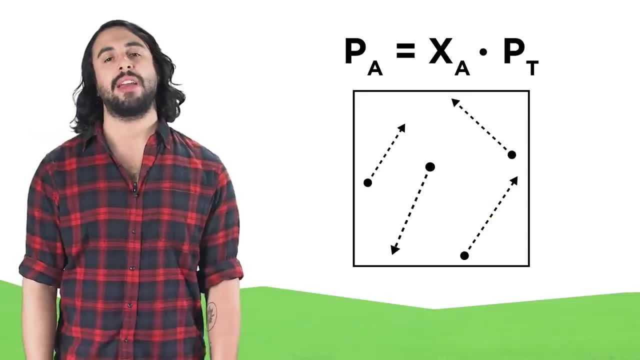 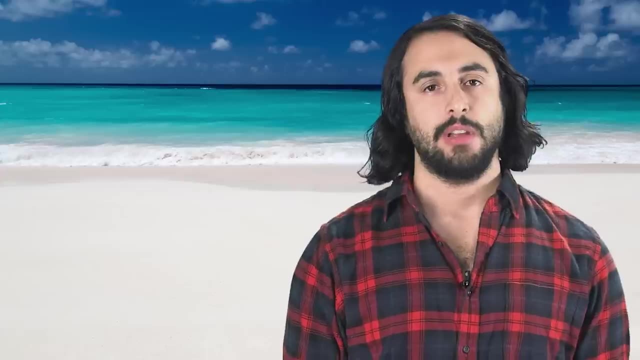 Again, this makes sense on the molecular level when we consider individual collisions occurring between the particles and the sides of the container and the fraction of these collisions that is represented by any individual substance. To see this demonstrated, let's say we capture a sample of earth's atmosphere at sea level. 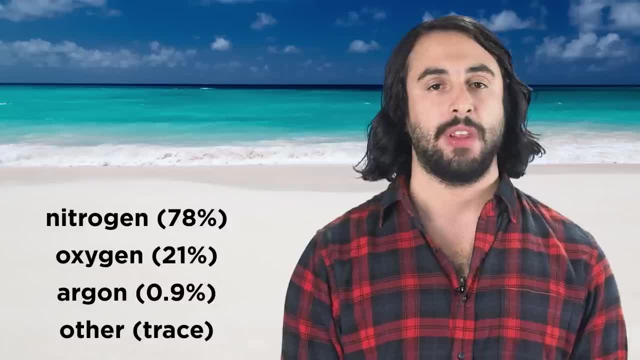 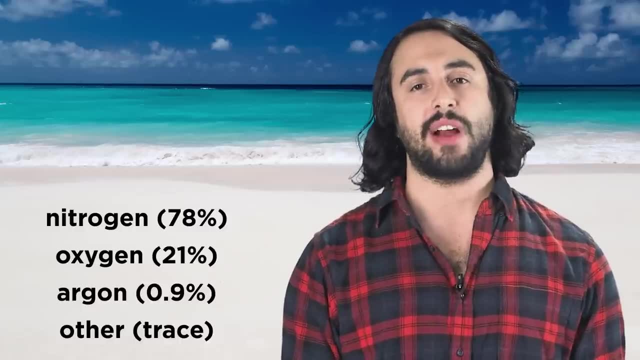 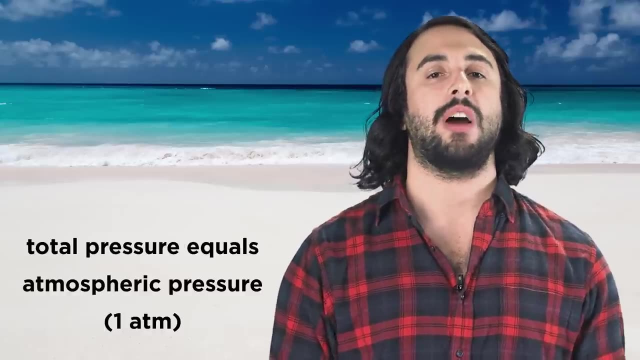 We know that there will be several different gases in the sample, as the atmosphere is comprised of nitrogen, oxygen and argon in roughly these quantities, plus trace amounts of a bunch of other things, and the sample as a whole exerts a pressure equal to atmospheric. 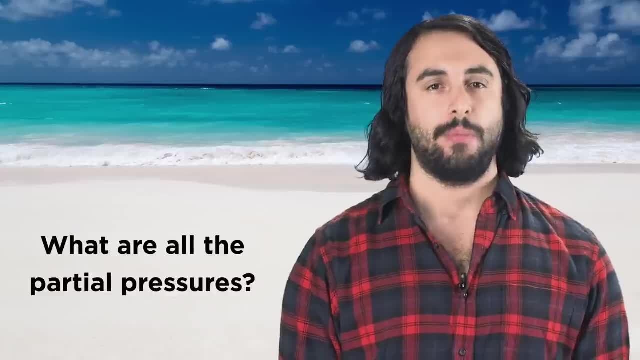 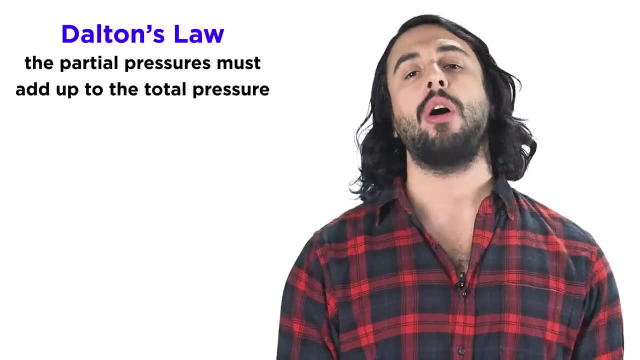 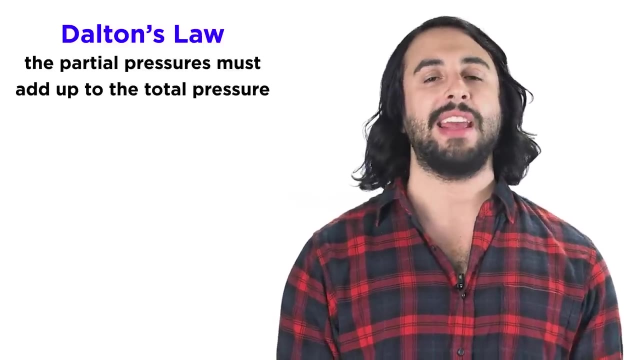 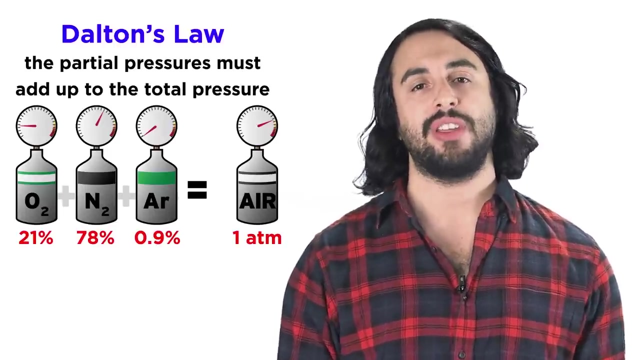 pressure or one atmosphere. But what contribution to this total is provided by each component of the gas? Recall that Dalton's law says that the sum of the partial pressures of the component gases in a mixture will be equal to the total pressure. That means that if we pretend the atmosphere is comprised of only these three gases, the 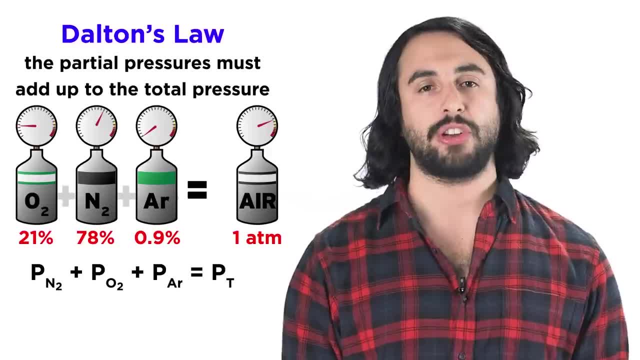 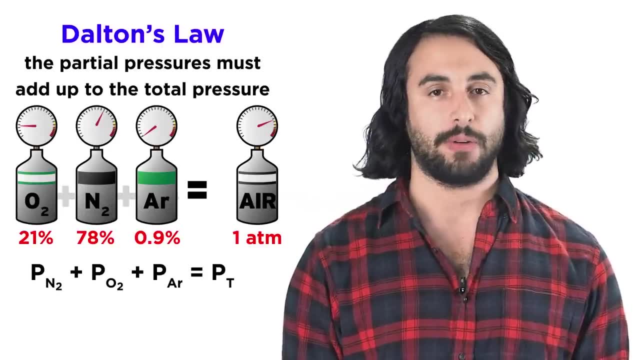 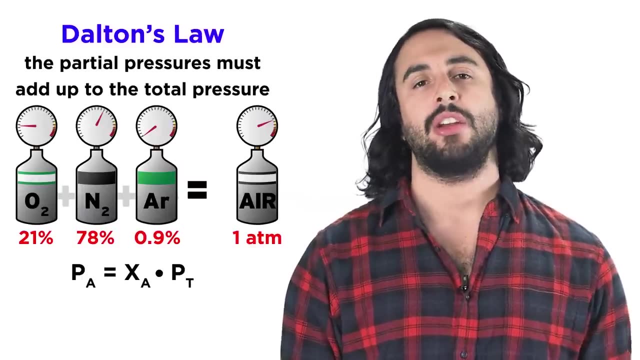 partial pressure of nitrogen, plus the partial pressure of oxygen, plus the partial pressure of argon will add up to atmospheric pressure. But how do we calculate the partial pressure of each gas? Well again, the partial pressure of a gas is related to the mole fraction of the gas. 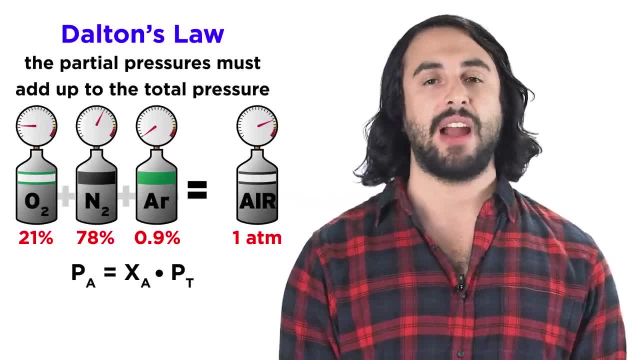 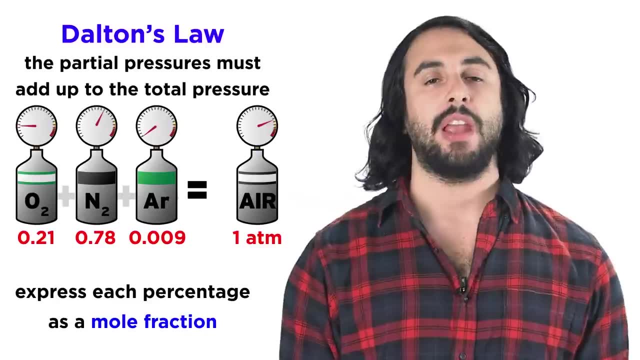 or the fraction of the mixture that gas represents by number of particles. This means we can take these percentages and divide them by a hundred in order to express them as mole fractions. This means we can take these percentages and divide them by a hundred in order to express them as mole fractions. 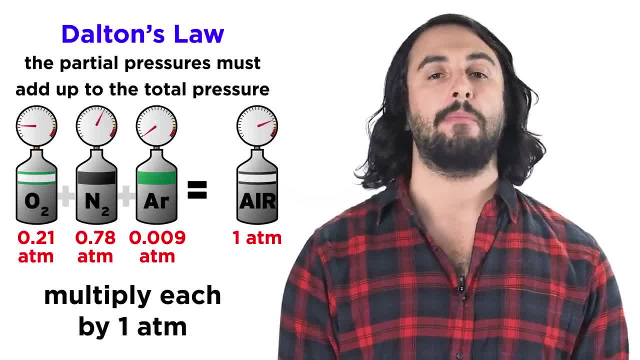 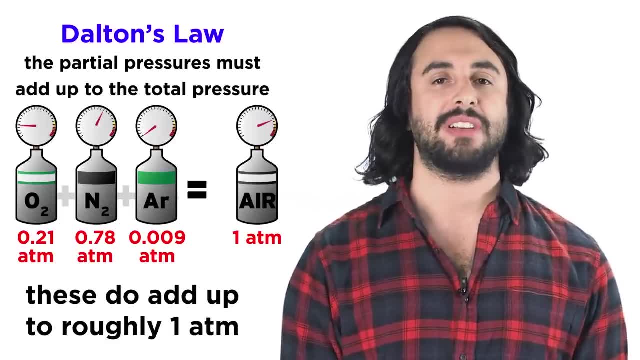 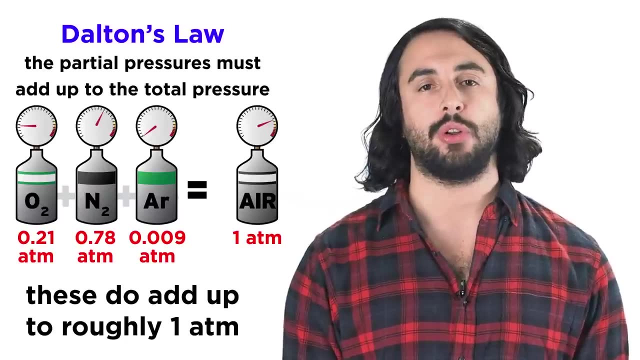 And then we can multiply each mole fraction by the total pressure to get the partial pressure of each substance. So it's quite simple to calculate the partial pressure of each gas in our sample, and we can see that these do add up to a total of one atmosphere, just as the individual percentages. 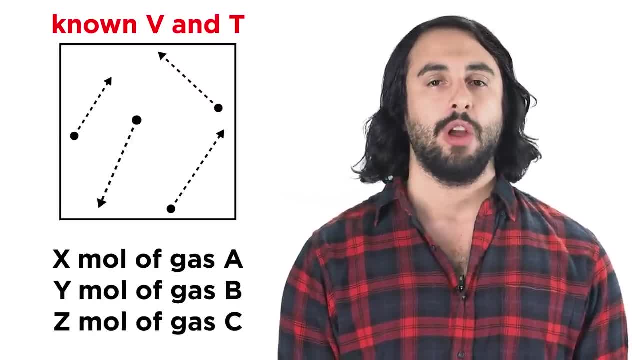 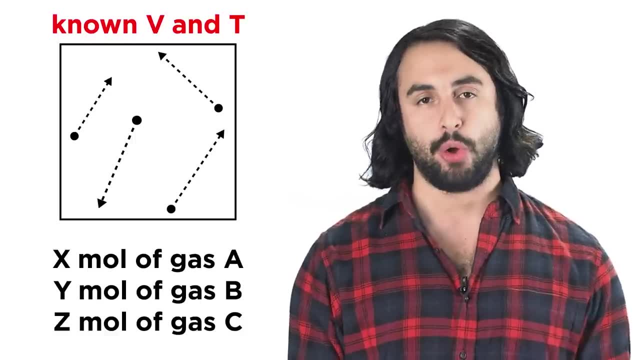 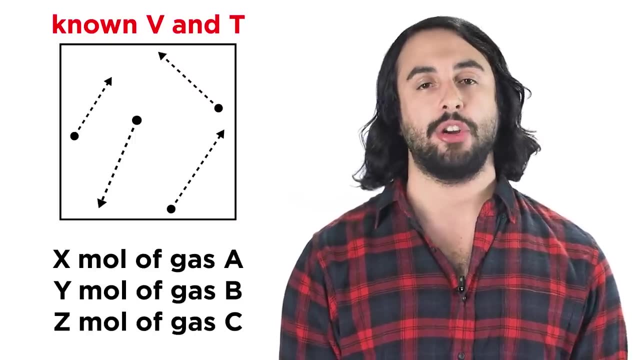 add up to one hundred percent. We can do trickier calculations as well by including other gas laws. Let's say we have quantities in moles of a few different gases and we place them into a vessel of known volume and at a known temperature. 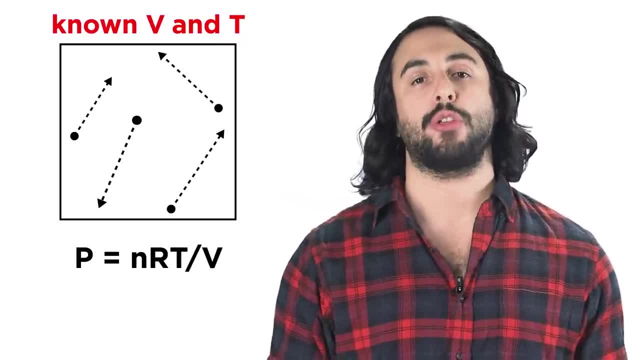 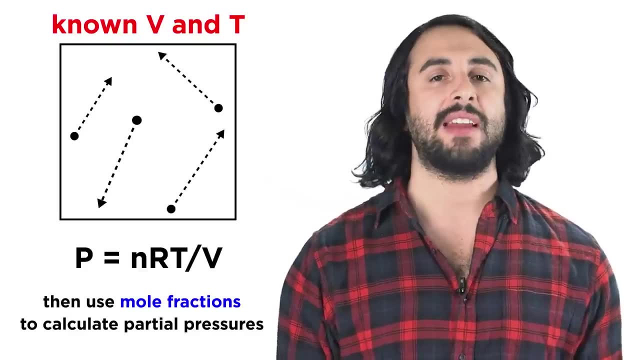